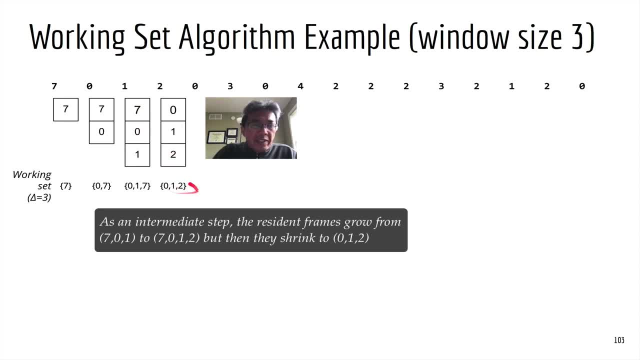 there, but then seven was removed because seven was not in a working set. the next reference to page zero triggers no page fault and again we need to update the working set. the working set stays the same. the next reference to page three will trigger another page fault and at that point page three will be added to. 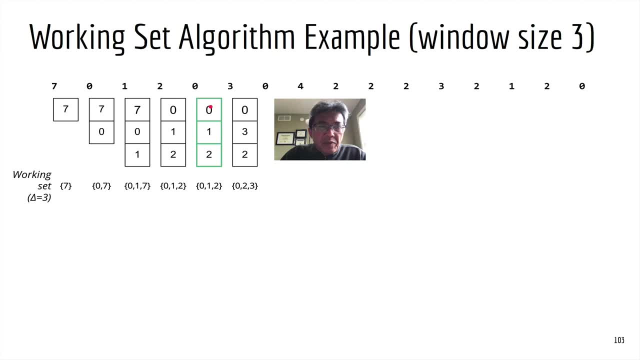 your frame. so the number of frames will grow from three to four. but again, when we update the working set, page one is not included in the working set. that's why page one was removed. the next reference to page zero does not trigger a page fault. but when we update the working set again, if you look back three frames, the working 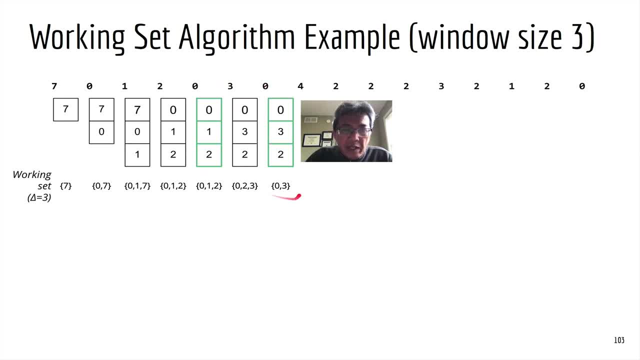 set includes only pages zero and three. that's why the working set is here. the next reference to page one is only effectively three frames that buy screen increased, increased the page change so get a more reference to page two and that's why that would be better. that's why every page. 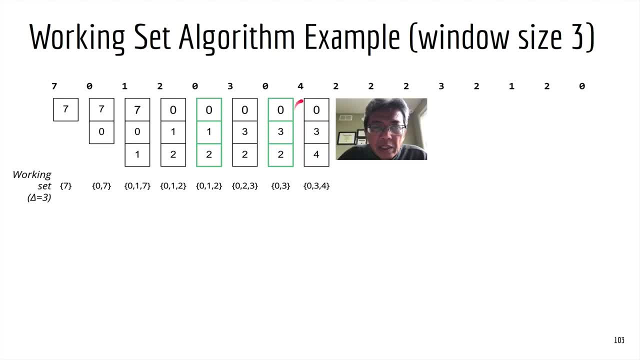 the next reference to page two, and that's why MIT version four is in 3, so we reference is to page four. that will trigger a page fault. and again, if you update the working set, the working set includes only pages zero, three and four. that's why two is kicked out. and if you 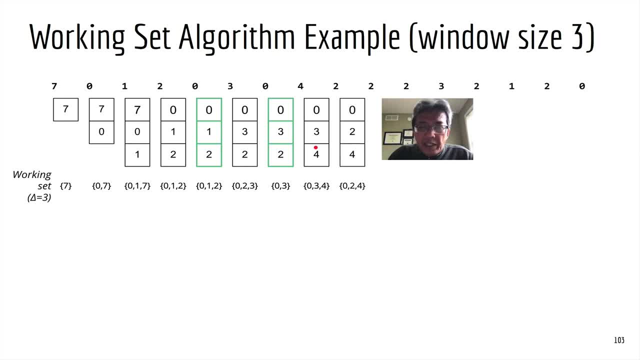 continue making the next reference to page two, another page fault. you update the working set and this is a new set of resident pages. the next reference to page two does not create a page fault, but now the working set again. if you look three frames back from the current time, 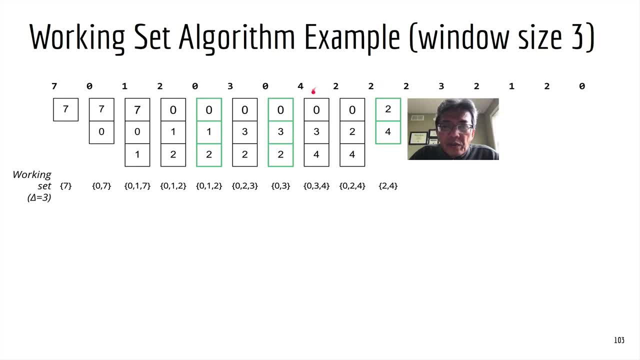 the working set includes only pages two and four. that's why page zero is kicked out and at this point the number of frames shrank from three to two. the next reference to page two does not trigger a page fault. but again, if you update the working set looking three frames back, the working set: 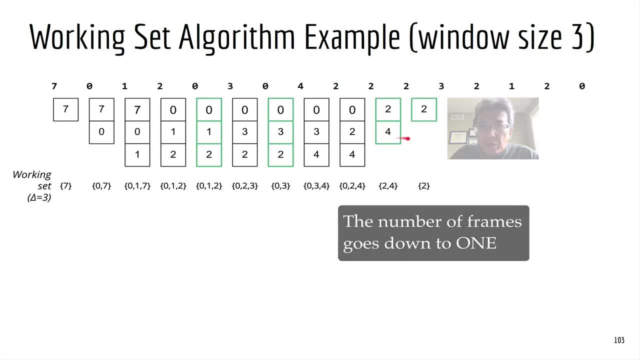 includes only page two. that's why page four is kicked out. so if you continue in this manner, then you will see the next few updates to the frames, to the resident frames will be shown here and now you can see that working set algorithm is indeed a dynamic algorithm because it will change the number of frames.